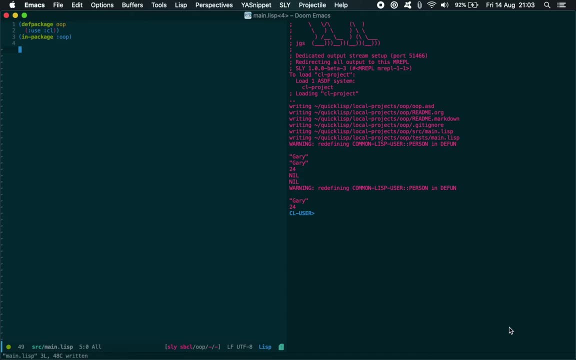 was selling functional programming short, because I was trying to come up with, you know, simple examples and academic examples of how to use things like map and reduce and lambda. And during the day I've had today, while I was teaching students this week, I've been teaching them about classes in JavaScript One. 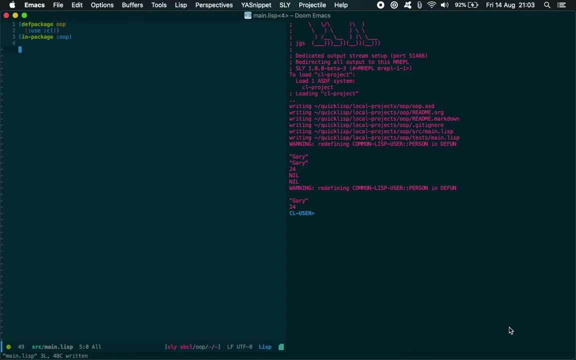 particular student came to me and said they didn't get JavaScript. Hmm, You know, that's fair, They come from a mathematical background, And so I had to go through some of the- the components of the lambda calculus, of course, from which 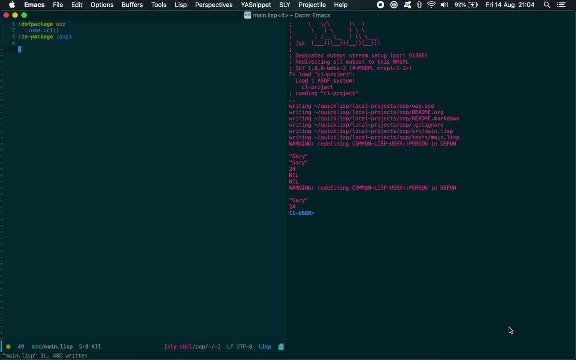 Common Lisp derives And we went through this and it made a lot more sense. I went away to the gym, I came back and then something hit me And although Common Lisp has an object system, it's got class. of course it is possible. 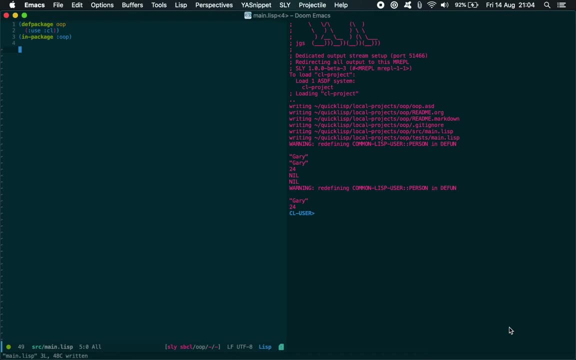 to build something that is arguably an object system. It's not going to be a great one. It's not particularly elegant. I'm not advocating that everybody go away and write their own object system or even use what I'm going to build here. 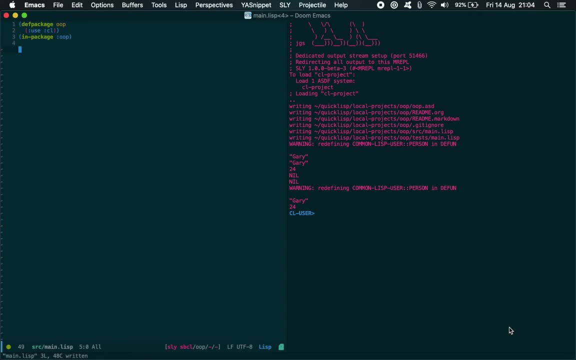 But I had success with a couple of students who understood functions but couldn't make the jump between functions and object orientation, And I came up with something I'm going to demonstrate here. So this is a perfect example of some parts of functional programming And, as the story goes, Lisp was used to create some of the 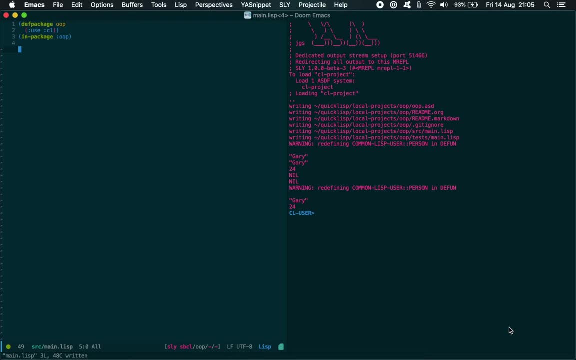 earliest object orientated inning, I believe, small-talk. Alan Kay built it in a version of Lisp. So we are going to have a wee go here and build our own object system using nothing but functions. so we're going to create a person and they take name and age. 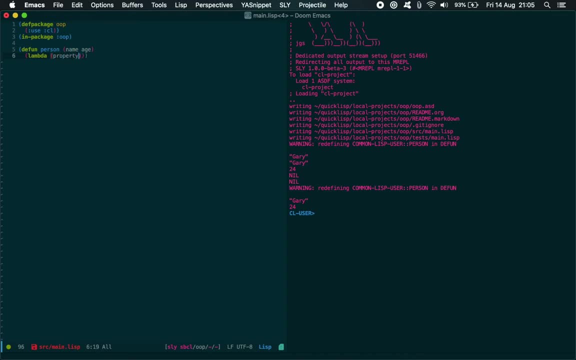 and it's going to return a lambda function which takes a parameter called property. and we're going to do a cond. I'm going to say string equals property. I'm going to say name. I'm going to return name: same here. we're going to say string property. 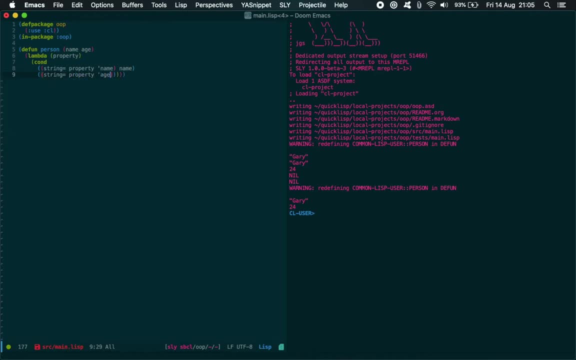 age age. we're going to compile that in and I'm going to create a little let here. P is person, Gary, he's going to be 24 and we're going to say: apply P actually print, apply P name print, apply P age. and then we've got Gary. 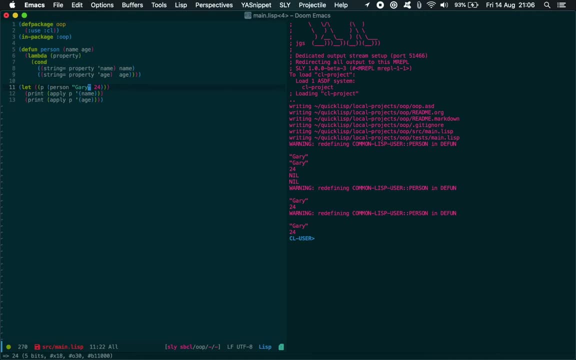 and 24. so we now have this function that is using a closure. so we're having a function that returns a function and that allows us to close over and capture. so we're going to say these values- name and age- so that's pretty cool. we have this function that 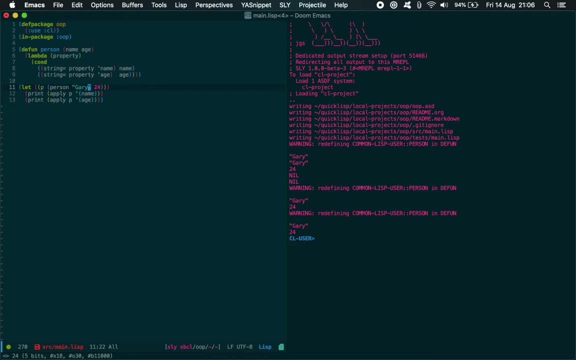 when called with particular parameters, will get the value stored in this. so this, arguably, is accessor properties. we go to the object, this function. we say we want the name and it gives us the value, or we want the age and it gives us the value. however, this is pretty ugly, so we're gonna write a convenience method. 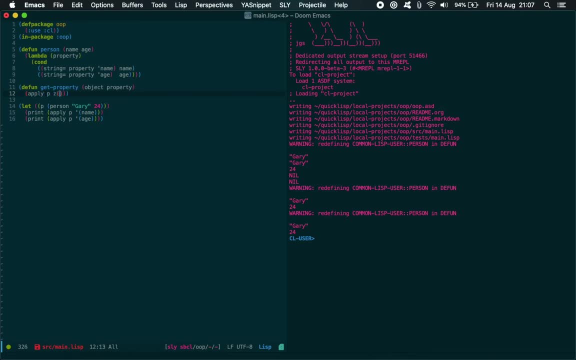 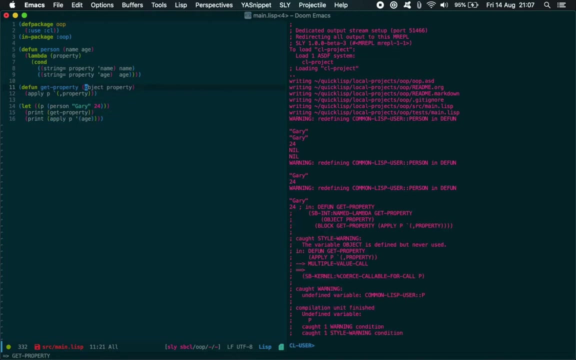 for. so now we're gonna say property, I need to compile this, of course, and that is apply object, not P. there we go. so I'm gonna make sure that's compiled in. we've redefined that. we've got no more. we've got no more. we've got no more. 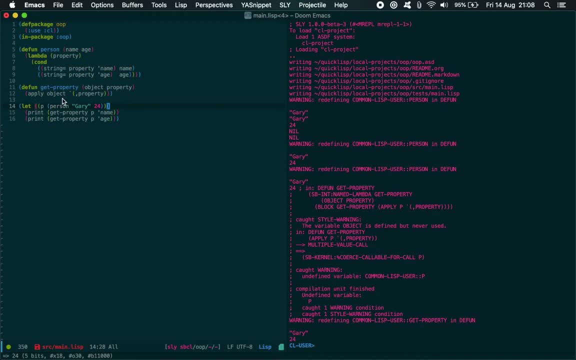 very little great. so if I run this now, we get Gary and 24, so this is much nicer. we're only using the supply in one place. now I'm gonna use that back ticket comma stuff to get that. so we now have this general get property function. but we can. 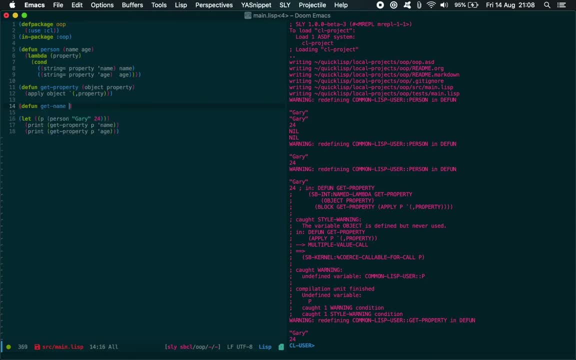 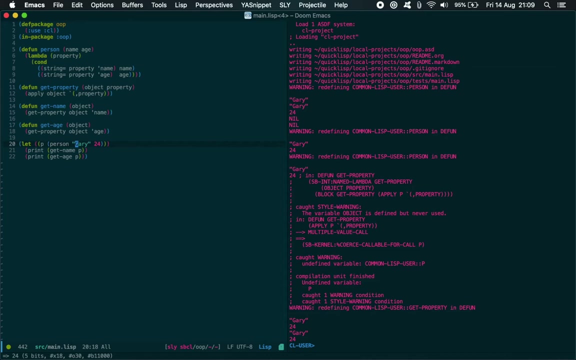 do better. you know, if you break this down it's going to be really easy. so if we put this in this? So now we've got these accessor methods for getName and getAge. My goodness, this heatwave in the pollen. it's really bad for my allergies, but never mind. 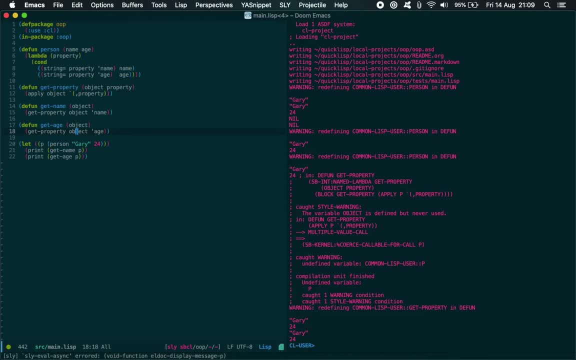 we will persevere. So this is really not a lot of code for what we've managed to achieve here. We're closing over a function and we're storing these properties in that function, and we can use accessor methods that we've created here and they get the values stored. 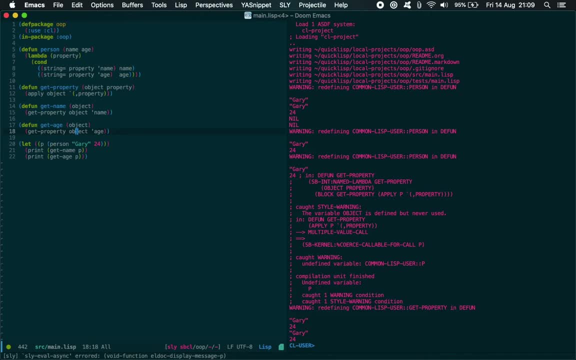 in that function, which is super cool. But this is only half an object system. it's like a read-only object system. After the object's been created, we cannot change these values, And that's unfortunate, but it is what it is. But we can work around this. 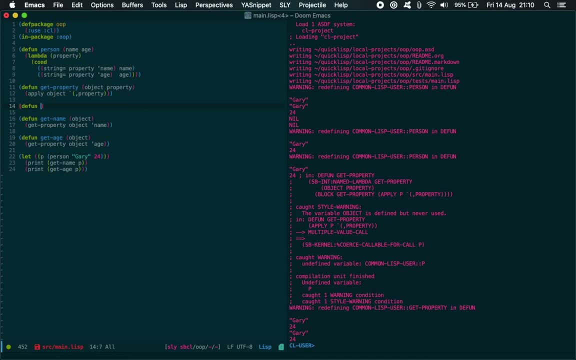 So we're going to get the property. so what we are going to do, I think, is We're going to use another cond here: String equals property name and we're going to say person and we're passing name. 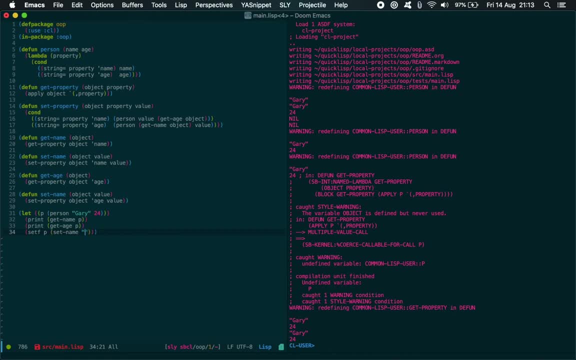 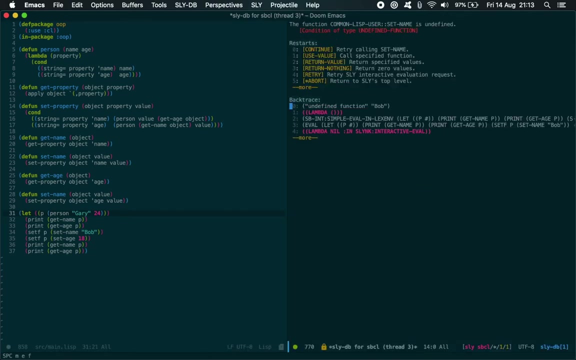 and we'll copy these two lines. so now, when we run this code, we have an error: set name as undefined. Of course I should compile that in. 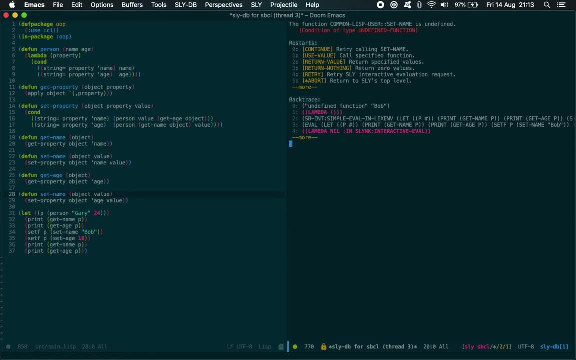 if I had it already, retry that. that's 4 invalid number of arguments. Of course that needs to be a P, of course. so let's abort that and just restart that. 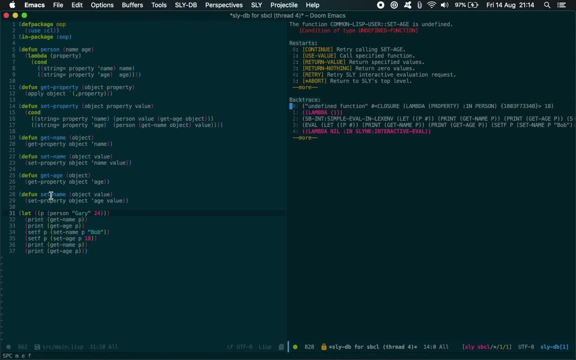 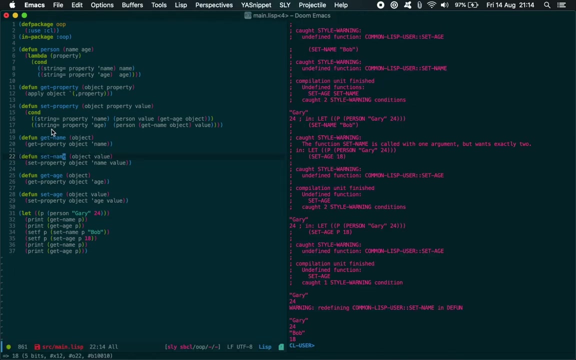 Set age as undefined. alright, sorry, I didn't notice that, so I'll have to redefine that one. There we go, Let's retry. There we go. a couple of errors, you know stupid little things, but we can see here. 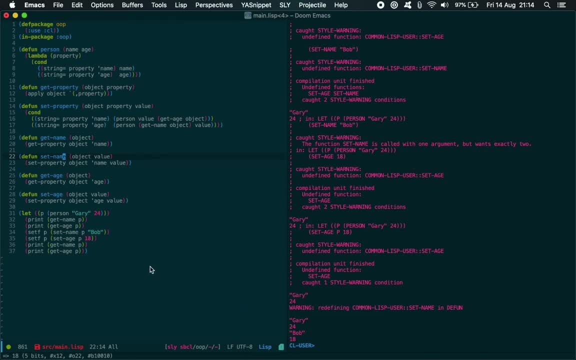 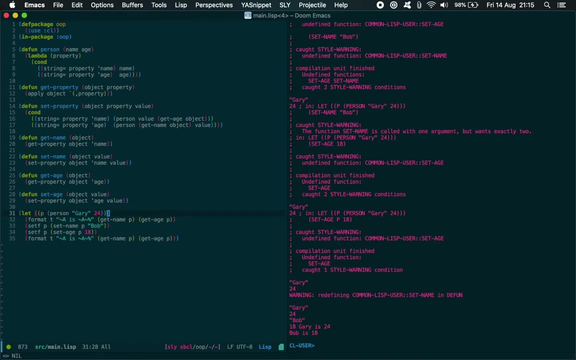 now in the right hand side we say Gary is 24, then we say Bob is 18, so let's phone up this just a little bit better. We'll get rid of those two. Alright, Save that and we'll do that. so we get yeah, okay, so that's just left over, because I didn't. 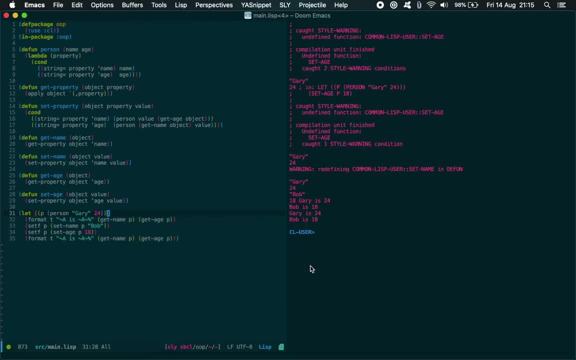 have the print light. so let's no the new light. there we go. I'll just clear that and we'll print that again. So Gary is 24,, Bob is 18.. We are able to set f our object here with the new values. it's a two-step process. 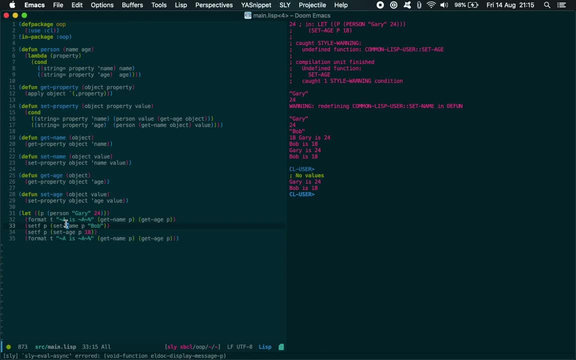 Not the most efficient in the world. of course, this is not a real object system, it is just a demonstration. but we can see here that all of the basic building blocks of an object orientation system, object orientated system, are here.